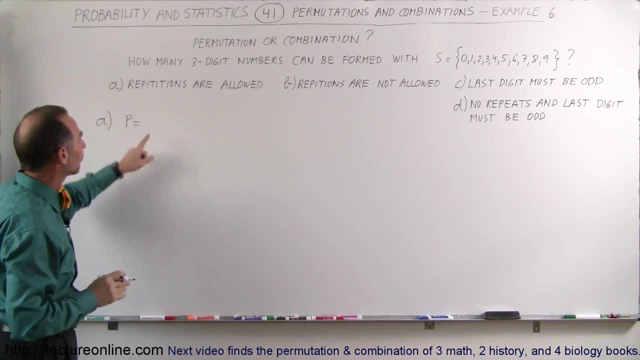 is going to be equal to. let's see here: how many options do you have for the first digit? Well, the first digit can be anything from one to nine, but not zero. That means there's no repetitions allowed. So what are the number of permutations in this case? 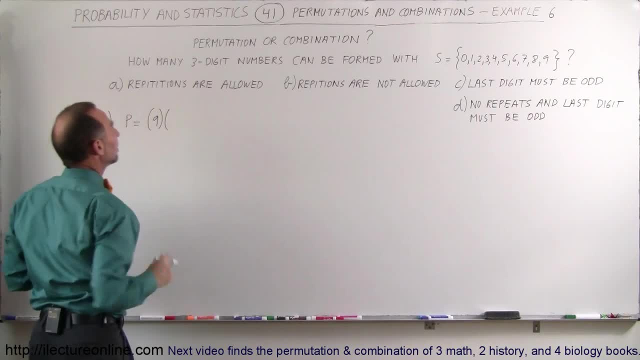 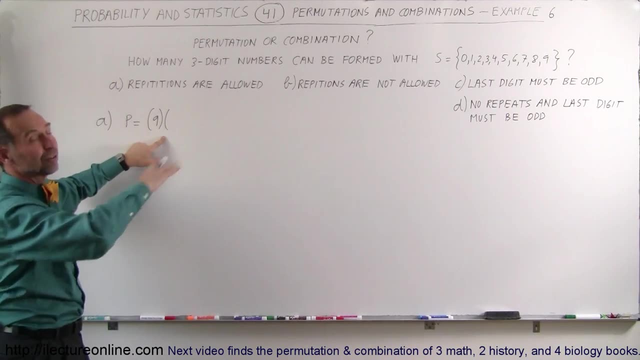 There's nine possibilities For the second digit. since repetitions are allowed there, you can have anything you picked before, plus any of the numbers from zero to nine. So therefore there's 10 possibilities. And again, for the third digit, there's no restrictions, So there's 10 different. 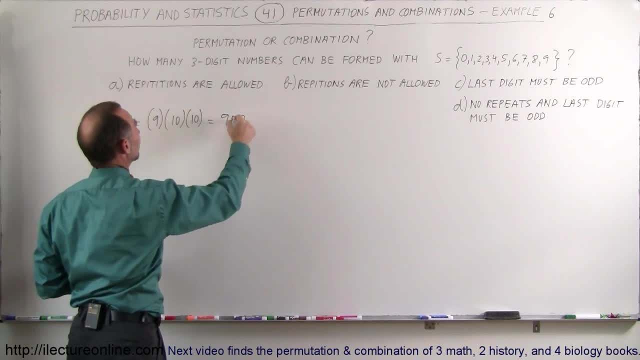 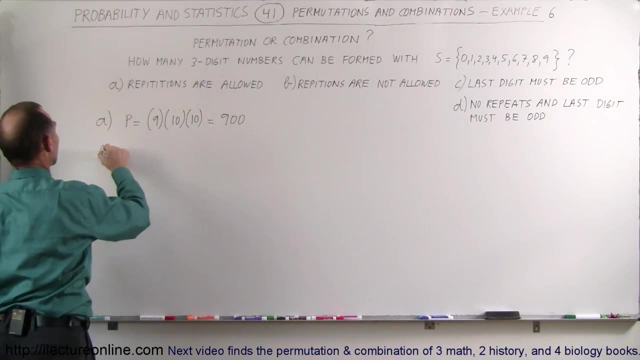 numbers you can pick there, And so in total we have 900 permutations when you want to make a three-digit number with the numbers from zero to nine. For part b, now we have a restriction: Repetitions are not allowed. So on the first try, on the first digit, we can only have nine possibilities because we can't pick. 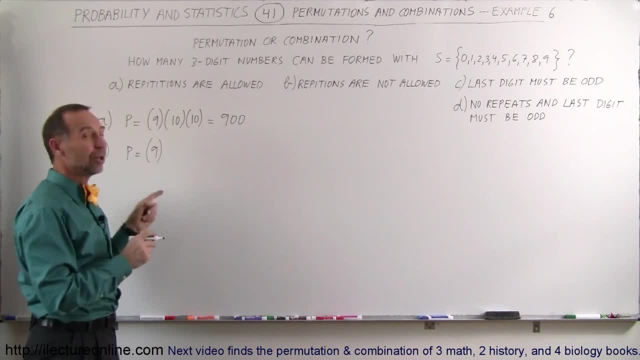 zero On the second one. since we already picked one number, we can't repeat that number, Since we had 10 before. now there's one less available, So you can only pick nine for the second digit And now, since you've picked two digits which cannot repeat, so two numbers already taken. 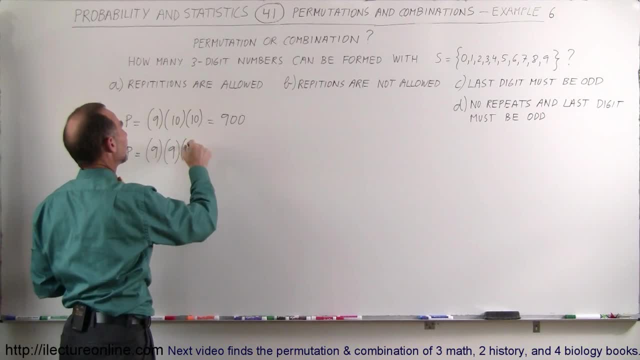 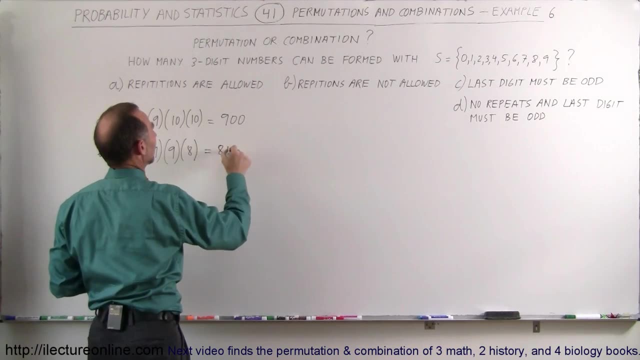 there's now only eight numbers left, And so therefore you can only put eight different possibilities for the third digit. So in this case, we can only pick one number. So we can only pick one number. So in this case you have nine times nine, which is 81 times eight, So that's 81 times. 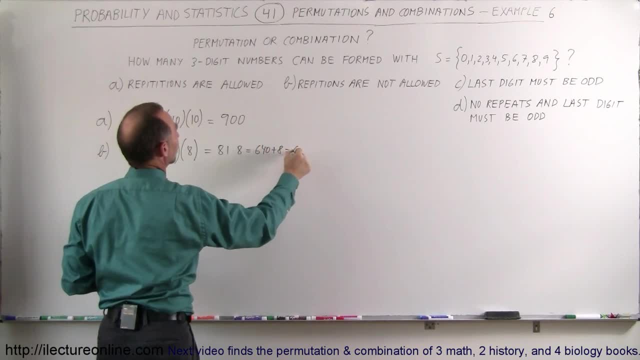 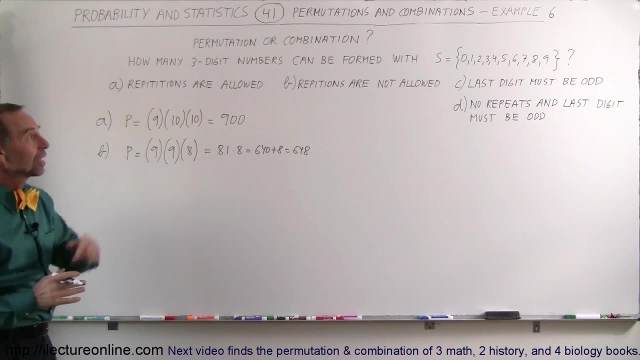 eight, which is equal to 640, plus eight, which is equal to 648 permutations, with three numbers coming up with a three-digit number. when you cannot use repeats On part c, the only restriction is that the last number must be odd. All right, so the number of permutations is nine for the first. 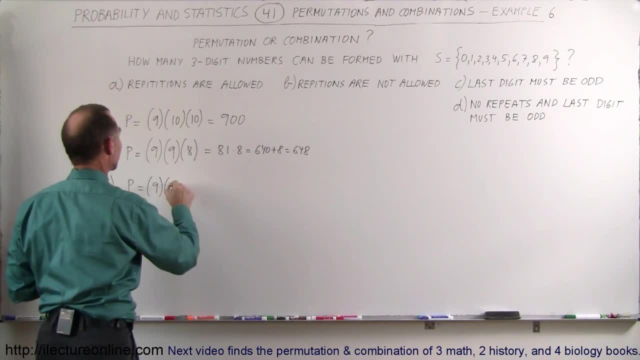 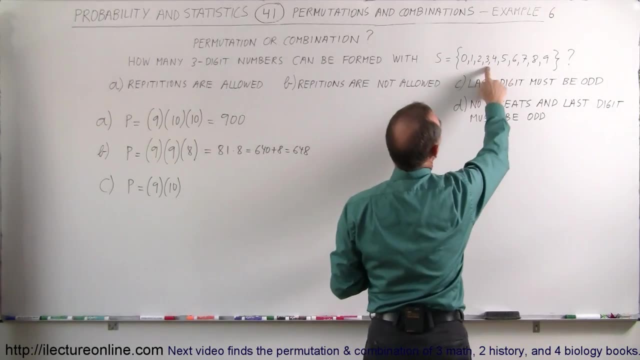 digit You can repeat, which means you have 10 possibilities for the third digit. So you can't repeat for the second digit, But for the third digit. it must be odd. It can be repeated, but it must be odd And we have one, two, three, four, five odds. So there's only five possibilities for 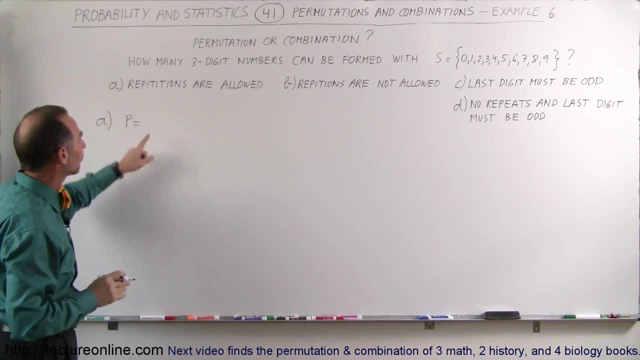 is going to be equal to. let's see here: how many options do you have for the first digit? Well, the first digit can be anything from one to nine, but not zero. That means there's no repetitions allowed. So what are the number of permutations in this case? 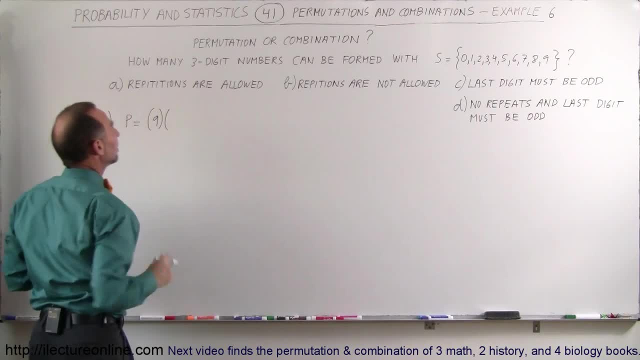 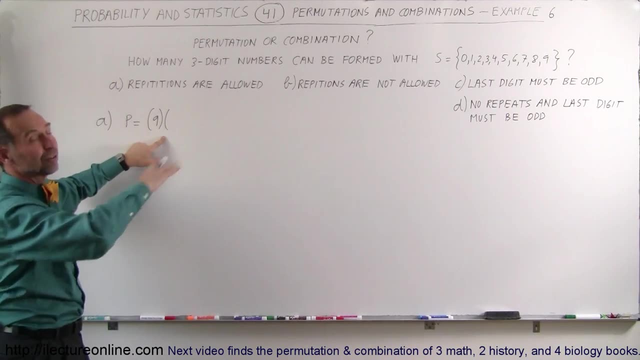 There's nine possibilities For the second digit. since repetitions are allowed there, you can have anything you picked before, plus any of the numbers from zero to nine. So therefore there's 10 possibilities. And again, for the third digit, there's no restrictions, So there's 10 different. 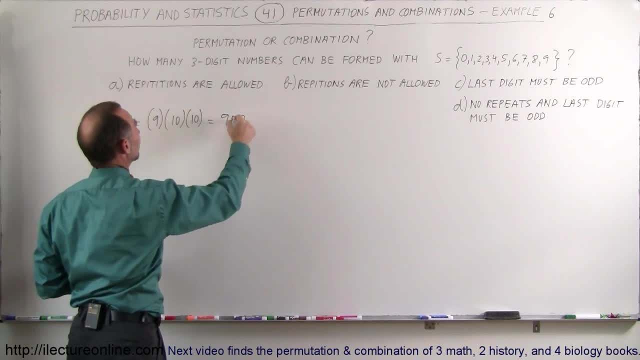 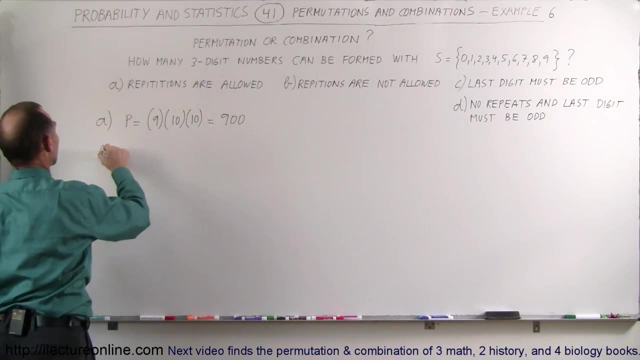 numbers you can pick there, And so in total we have 900 permutations when you want to make a three-digit number with the numbers from zero to nine. For part b, now we have a restriction: Repetitions are not allowed. So on the first try, on the first digit, we can only have nine possibilities because we can't pick. 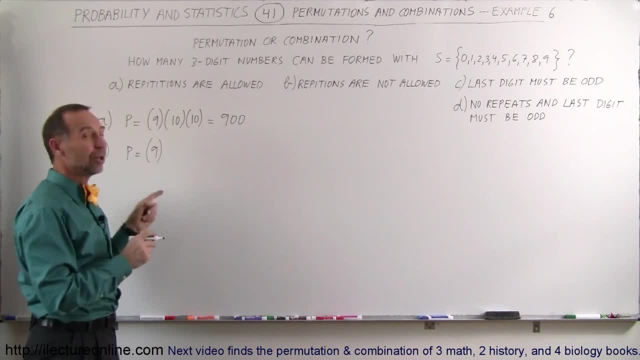 zero On the second one. since we already picked one number, we can't repeat that number, Since we had 10 before. now there's one less available, So you can only pick nine for the second digit And now, since you've picked two digits which cannot repeat, so two numbers already taken. 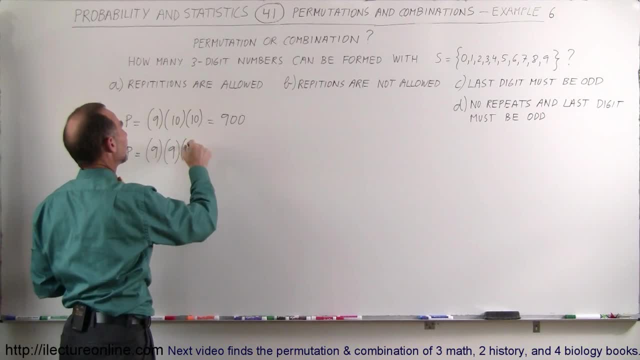 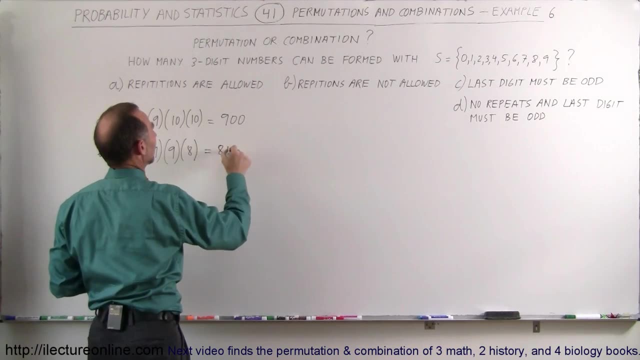 there's now only eight numbers left, And so therefore you can only put eight different possibilities for the third digit. So in this case, we can only pick one number. So we can only pick one number. So in this case you have nine times nine, which is 81 times eight, So that's 81 times. 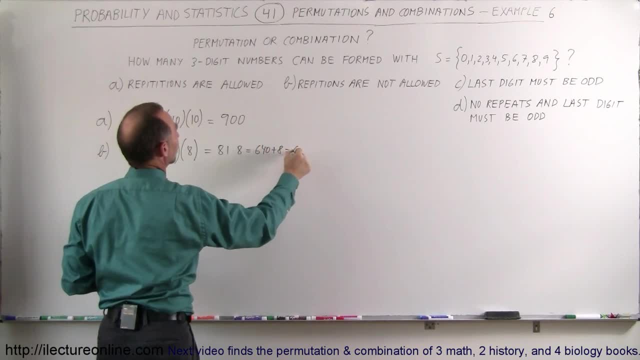 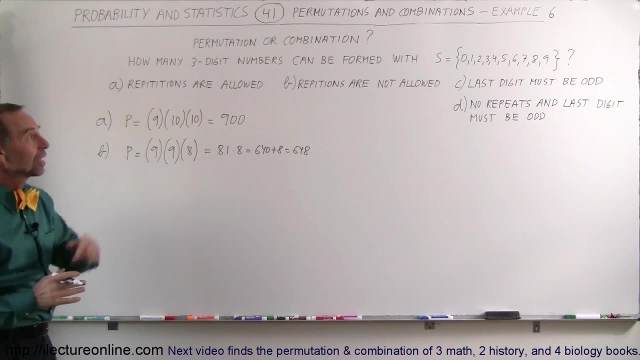 eight, which is equal to 640, plus eight, which is equal to 648 permutations, with three numbers coming up with a three-digit number. when you cannot use repeats On part c, the only restriction is that the last number must be odd. All right, so the number of permutations is nine for the first. 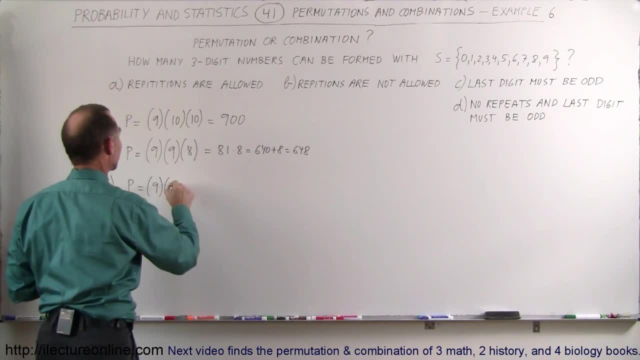 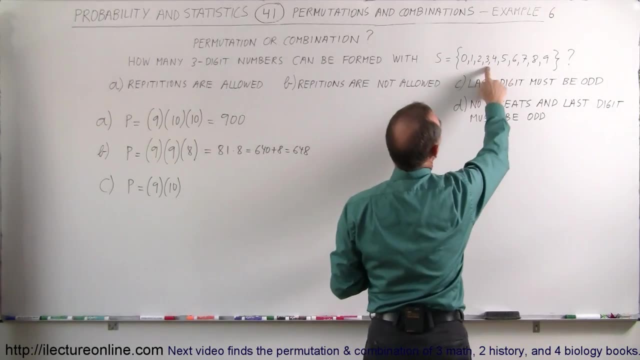 digit You can repeat, which means you have 10 possibilities for the third digit. So you can't repeat for the second digit, But for the third digit. it must be odd. It can be repeated, but it must be odd And we have one, two, three, four, five odds. So there's only five possibilities for 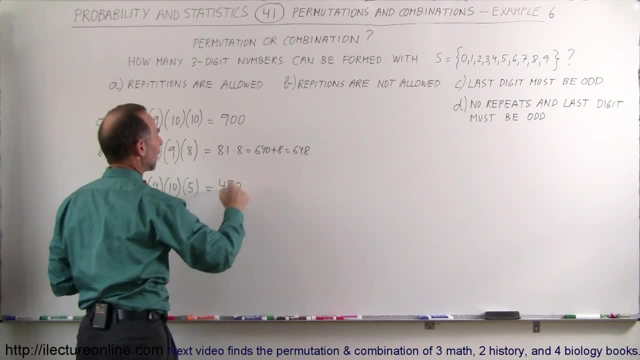 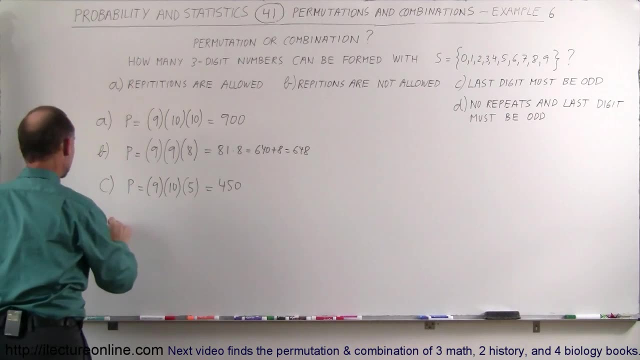 the third digit, That's 50 times nine or 450 possibilities. Now what about if you cannot have any repeats and the last digit must be odd? So part d, the number of permutations, is equal to again for the first one. you can have nine possibilities. So 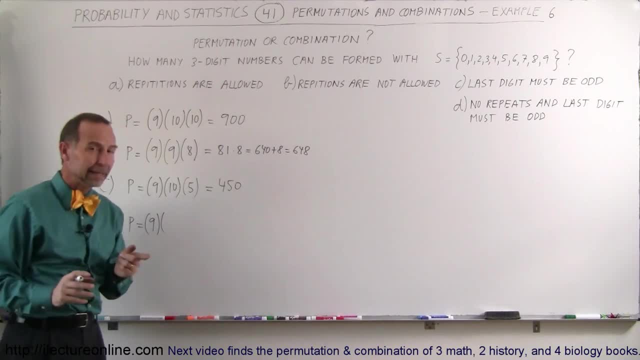 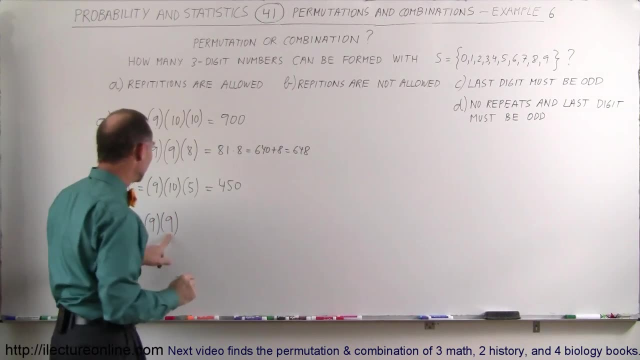 nine, because it cannot be a zero For the second digit, since you cannot have a repeat other than that. it can be anything you want. You can have a possible nine numbers you can put in here, because you can't repeat whatever you had in the first one, Now in the last one- it must be odd, But in 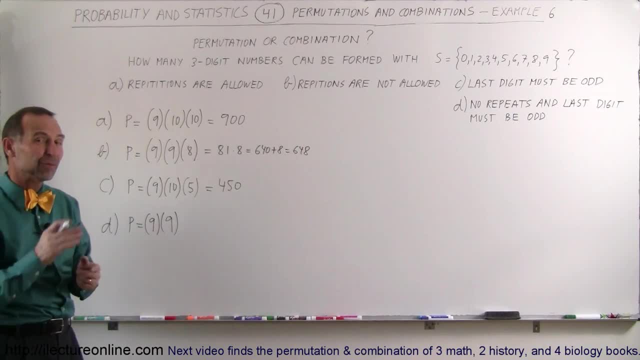 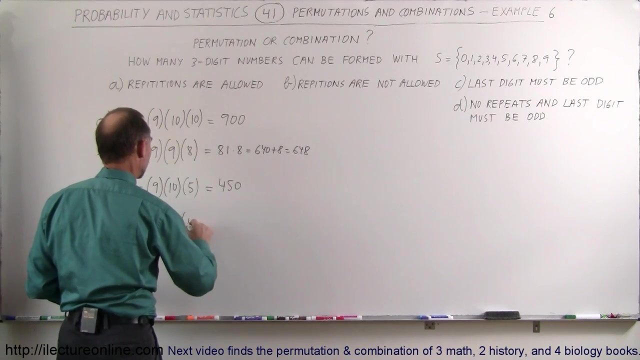 addition to that, you can already have taken anywhere from zero to two odds. So you only have either five possibilities, four possibilities or three possibilities, depending upon how many you picked here. If you already picked, if you picked no odds, then you can have five more possibilities at the end. So that's. 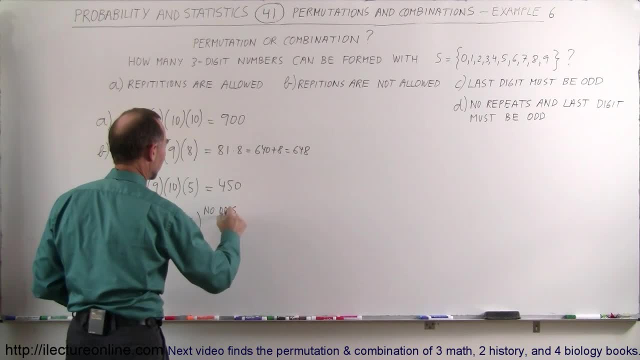 when you have the case with no odds were picked before, And so therefore, it's nine times nine, which is 81 times five, which is going to be 455, I believe right. So let's see here: That's 45, 450.. Oh, 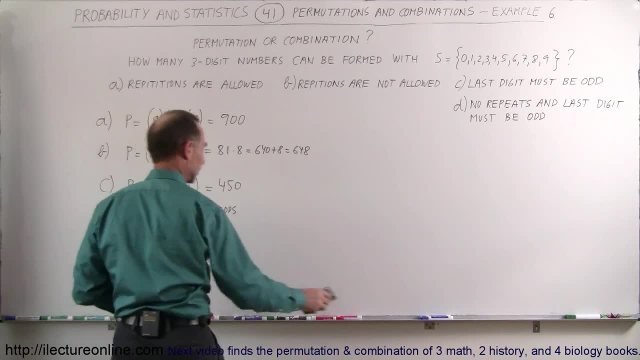 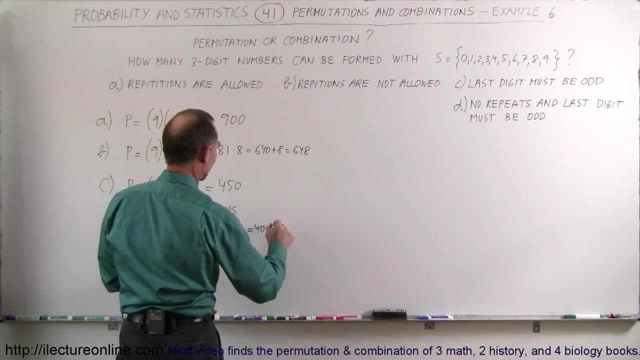 let me try that again. I don't think that's correct. So nine times nine is 81 times five. five times eight is 400.. Five times one is five. that's equal to 405.. That's a lot better. So no odds were. 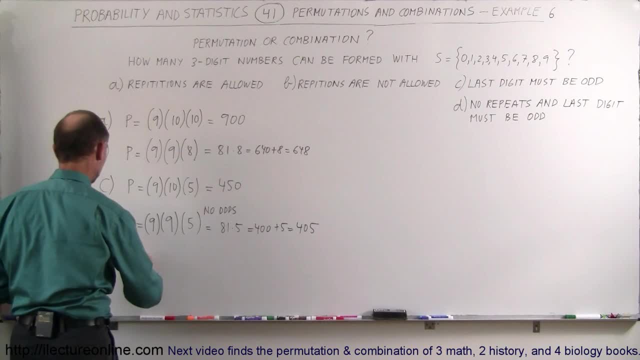 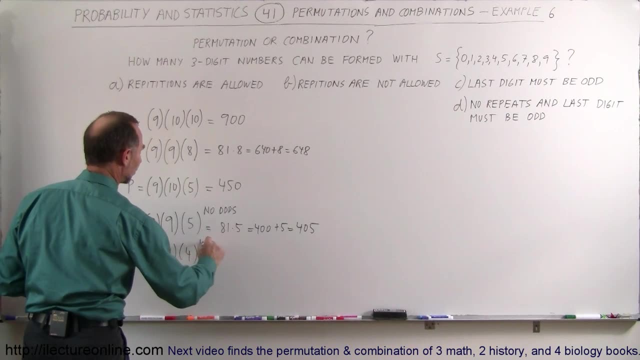 picked four and five permutations. But what if one of the first ones was an odd? So we have nine possibilities there, nine possibilities there, but now you'll have four possibilities if one odd was picked before. So in this case you're going to have 81 times four. four times eight is 320, that. 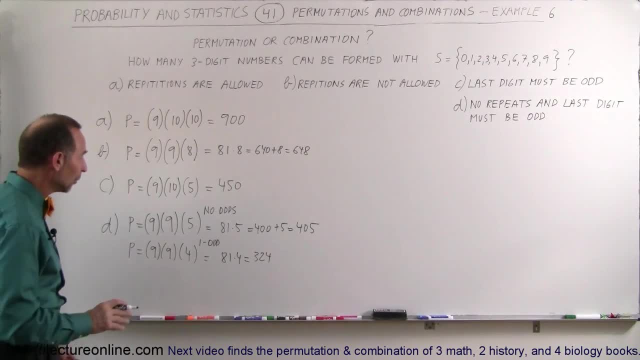 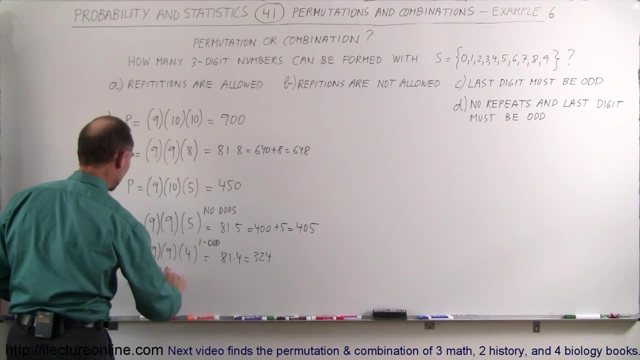 would be 324 permutations. And finally, what if the first two numbers were odds? then how many permutations do you have? So permutations equal to nine times nine. that will not change. But now you'll have three possibilities left, because two would already be taken. you can't repeat So. 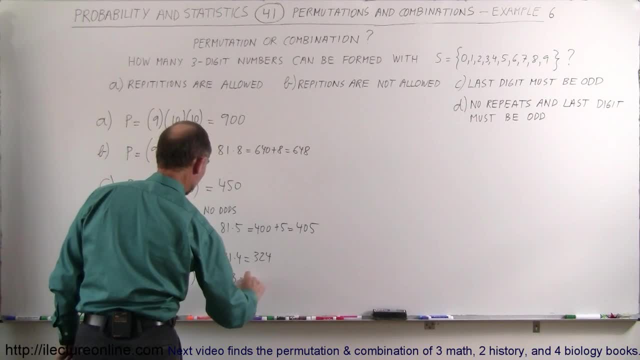 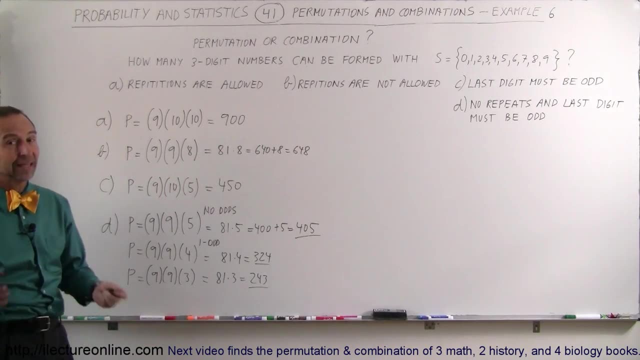 therefore, we have 81 times three, which is equal to 243 permutations. So there we have three possible answers, depending upon what happened before, And that's how we do that problem. 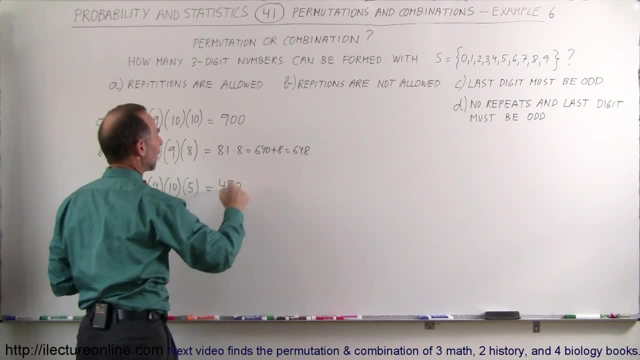 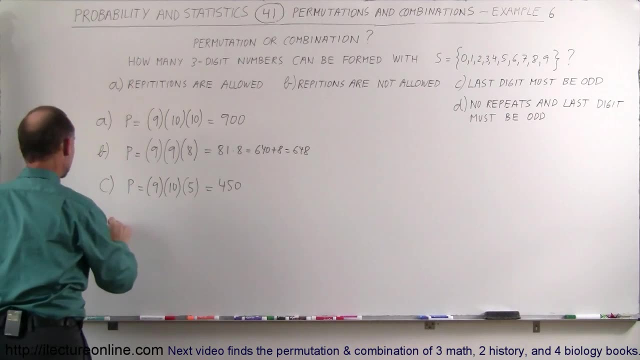 the third digit, That's 50 times nine or 450 possibilities. Now what about if you cannot have any repeats and the last digit must be odd? So part d, the number of permutations, is equal to again for the first one. you can have nine possibilities. So 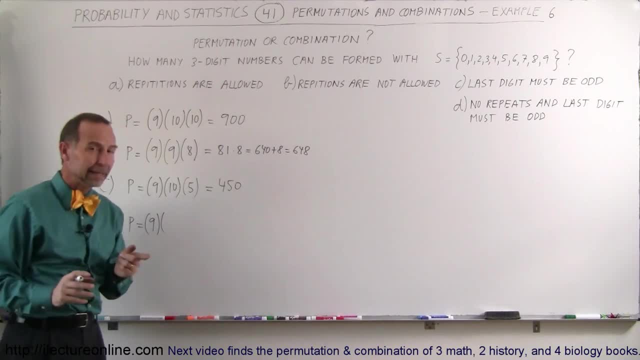 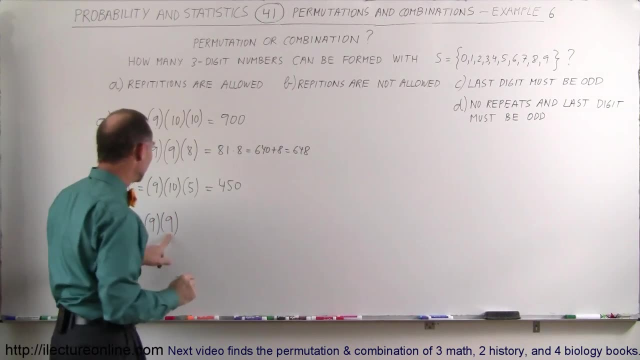 nine, because it cannot be a zero For the second digit, since you cannot have a repeat other than that. it can be anything you want. You can have a possible nine numbers you can put in here, because you can't repeat whatever you had in the first one, Now in the last one- it must be odd, But in 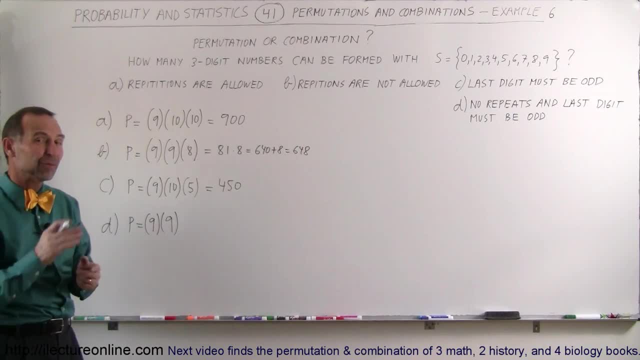 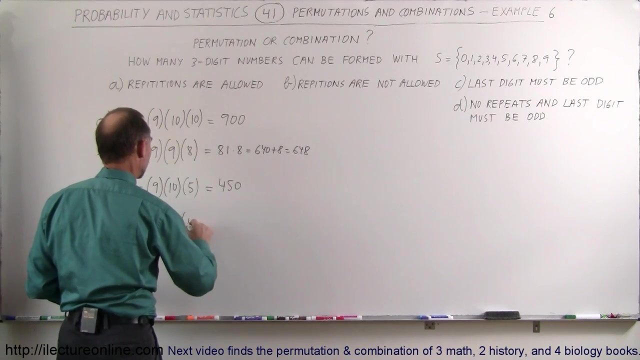 addition to that, you can already have taken anywhere from zero to two odds. So you only have either five possibilities, four possibilities or three possibilities, depending upon how many you picked here. If you already picked, if you picked no odds, then you can have five more possibilities at the end. So that's. 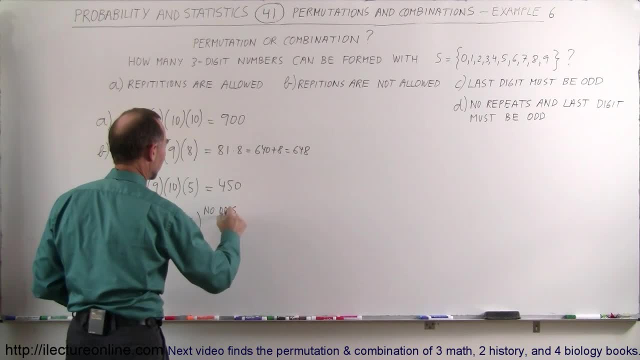 when you have the case with no odds were picked before, And so therefore, it's nine times nine, which is 81 times five, which is going to be 455, I believe right. So let's see here: That's 45, 450.. Oh, 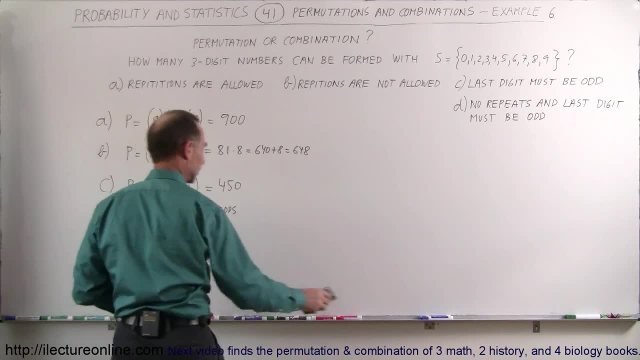 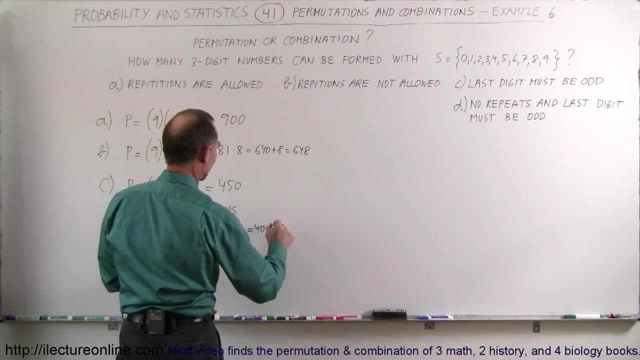 let me try that again. I don't think that's correct. So nine times nine is 81 times five. five times eight is 400.. Five times one is five. that's equal to 405.. That's a lot better. So no odds were. 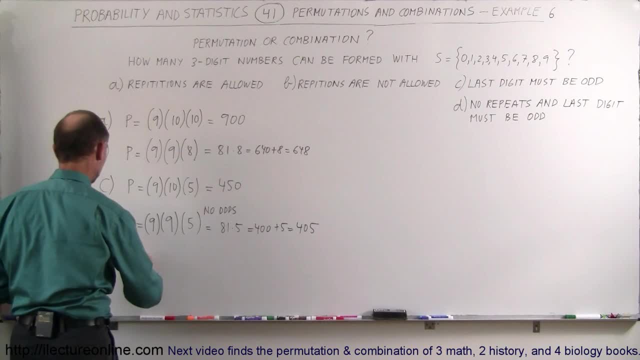 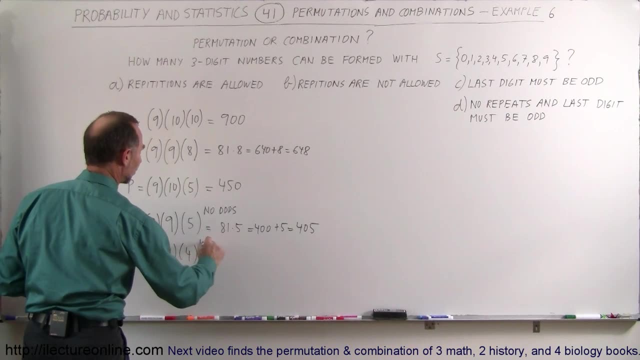 picked four and five permutations. But what if one of the first ones was an odd? So we have nine possibilities there, nine possibilities there, but now you'll have four possibilities if one odd was picked before. So in this case you're going to have 81 times four. four times eight is 320, that. 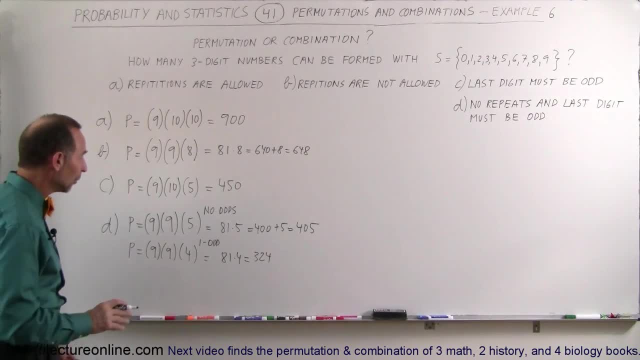 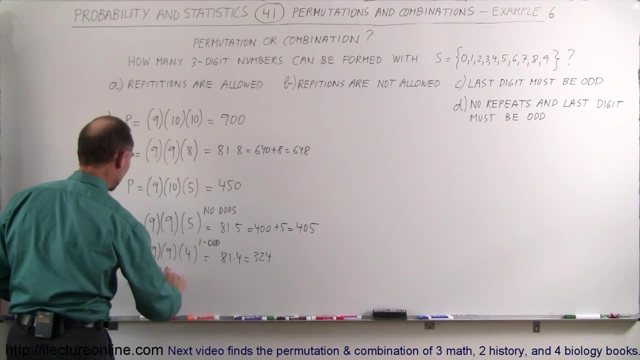 would be 324 permutations. And finally, what if the first two numbers were odds? then how many permutations do you have? So permutations equal to nine times nine. that will not change. But now you'll have three possibilities left, because two would already be taken. you can't repeat So. 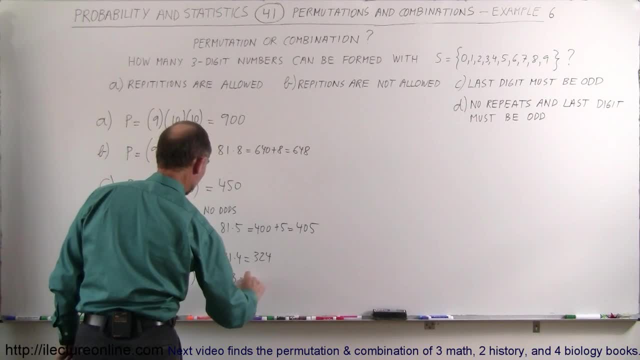 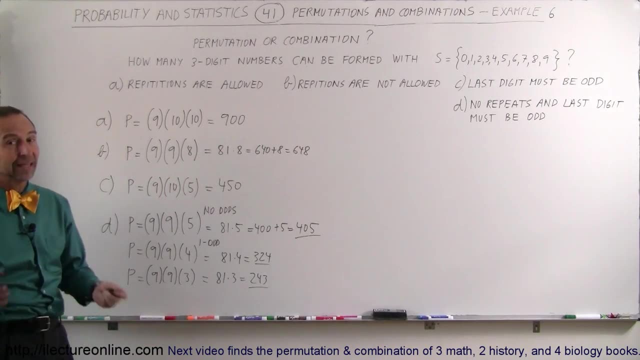 therefore, we have 81 times three, which is equal to 243 permutations. So there we have three possible answers, depending upon what happened before, And that's how we do that problem.